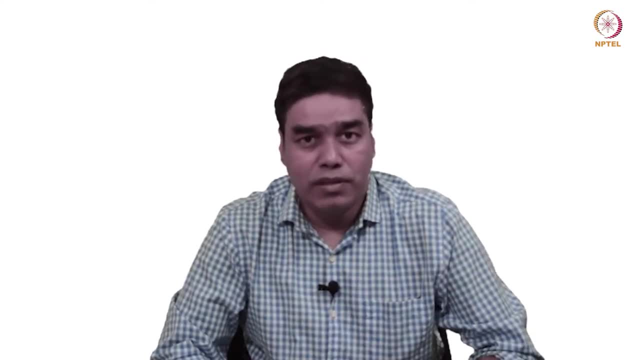 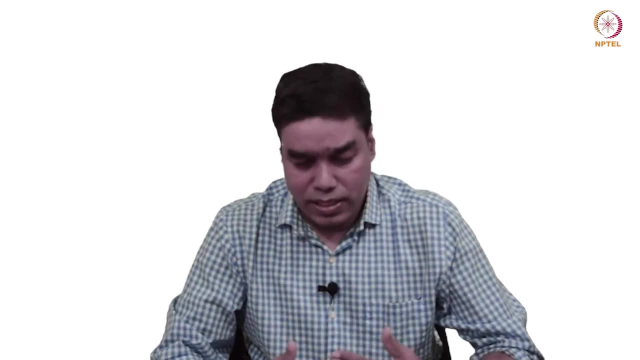 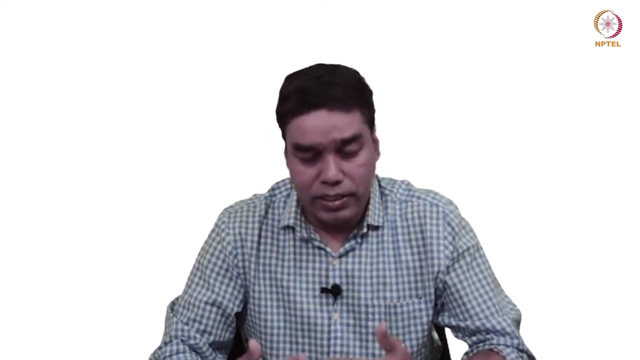 then, in past few classes, we have been talking about this compaction process with regard to shaping the powder into a particular form. right, and we have seen with regard to shaping the powder. We have seen that the powder can be shaped by different processes depending on the complexity. 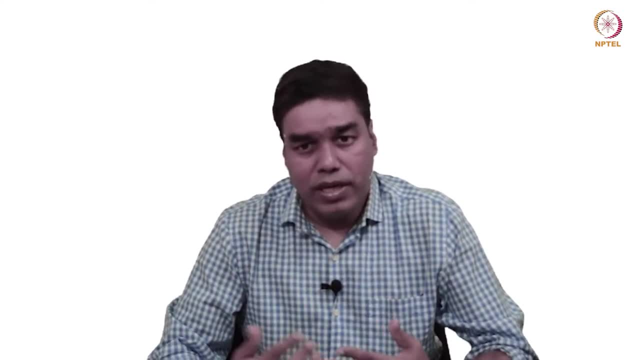 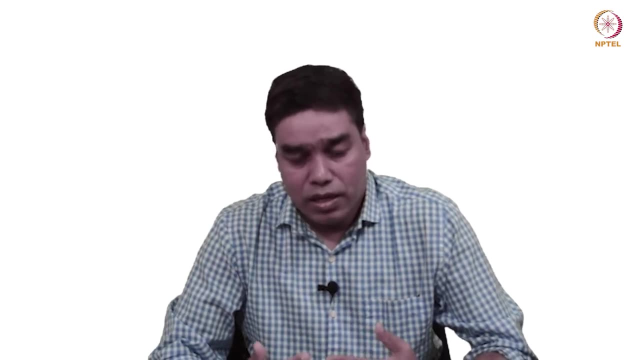 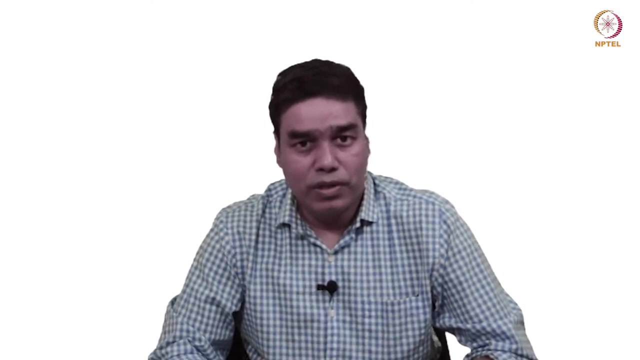 of the shape. If it is a simple shape, we can use uniaxial pressing, for example. Then we have talked about some other processes, other shaping processes also, which can deal with more complex shapes. For example, we talked about the powder injection molding. 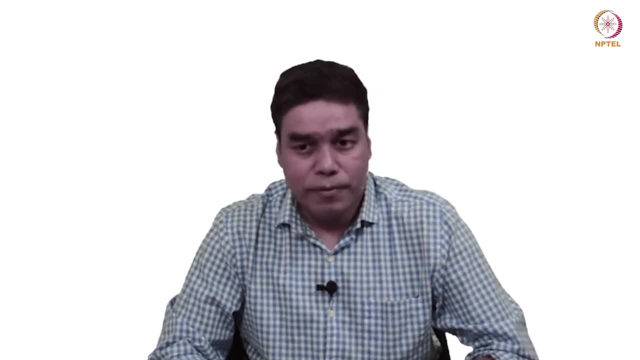 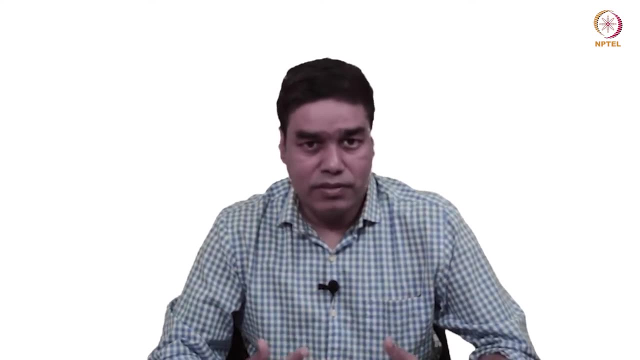 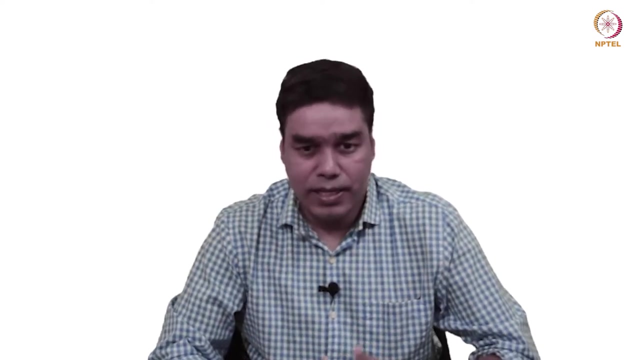 which can deal with 3D complex shapes. And then we have also spoken about the cold isostatic pressing, which is a more uniform pressing technique which is much effective compared to the uniaxial pressing, because here the pressure can be applied uniformly in all directions and, as a result, the compact 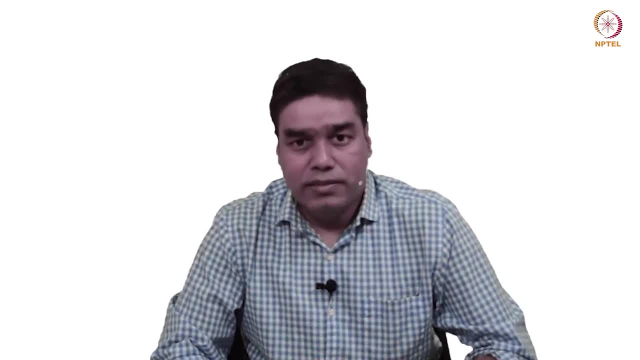 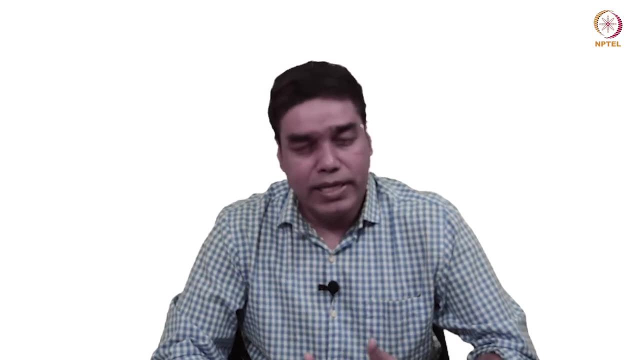 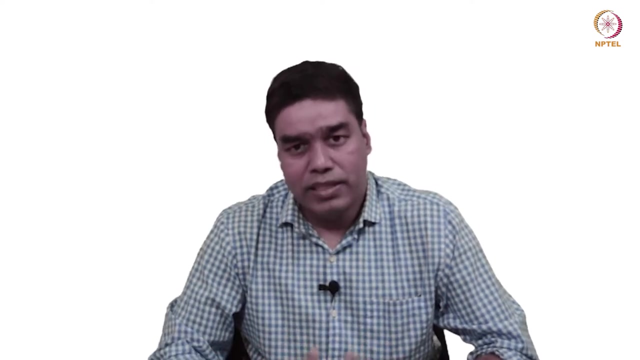 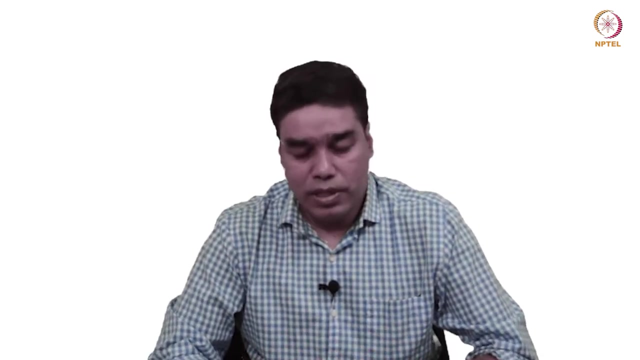 is uniform in terms of the density which is achieved After the compaction process. then we also talked about the slurry techniques to make other kinds of shapes, for example flat, thin products or long products. For such kind of shapes slurry techniques are more suitable. We have discussed that also in detail in past. 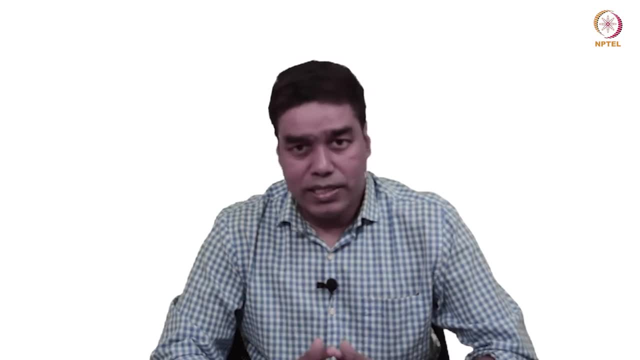 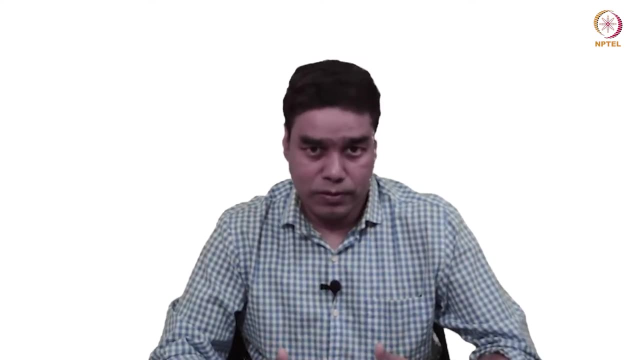 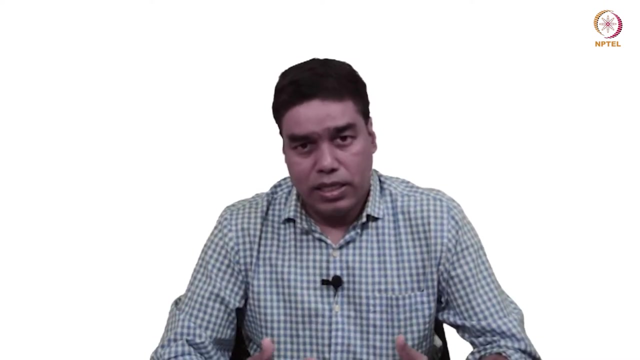 couple of classes. So now we are in a stage where the green compact is ready. We have presented the process of, mustn't it? So let us take a look at the final process. So this is the final stage where the green compact is to be processed, and the porosity 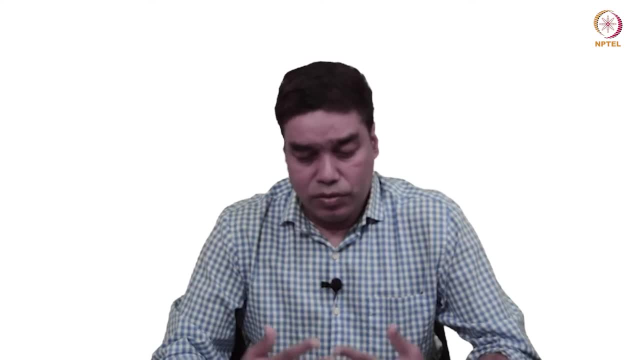 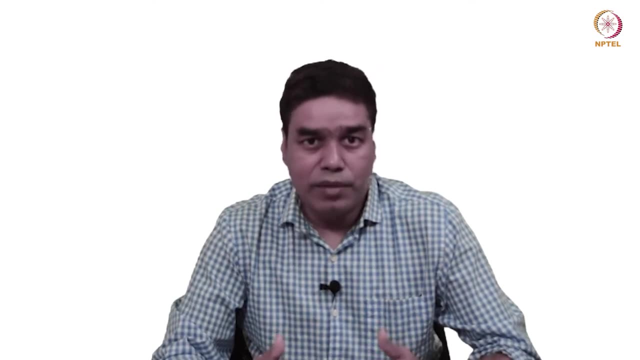 is left behind are to be closed to finally come up with a fully dense product. ok, So this is the final stage where the ultimate densification will take place, right? So that is the process that we are going to talk about. 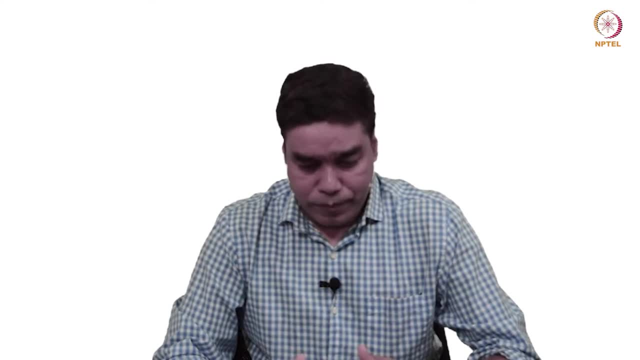 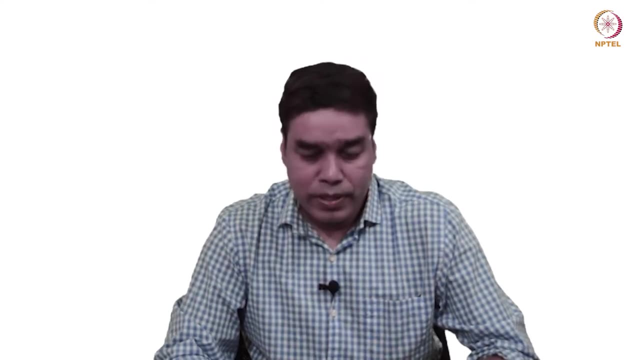 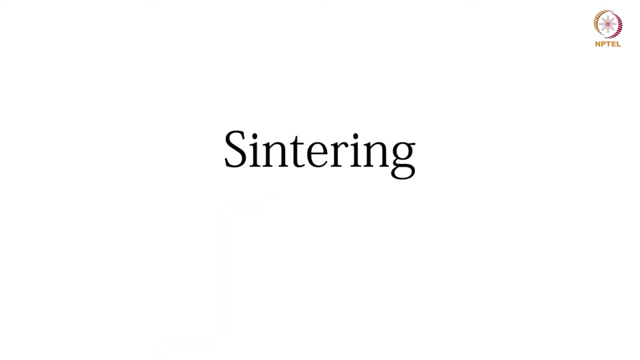 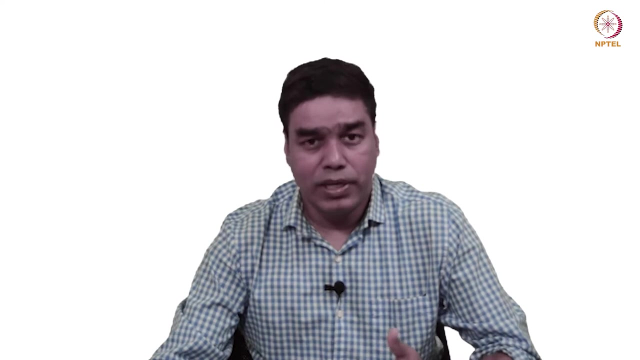 talk about from now onwards as to how this densification takes place and what are the process details. ok, So the process that we are talking about is called sintering and, as I said, this is the final step in the powder metallurgy process to densify the compact and obtain a fully dense product. ok, 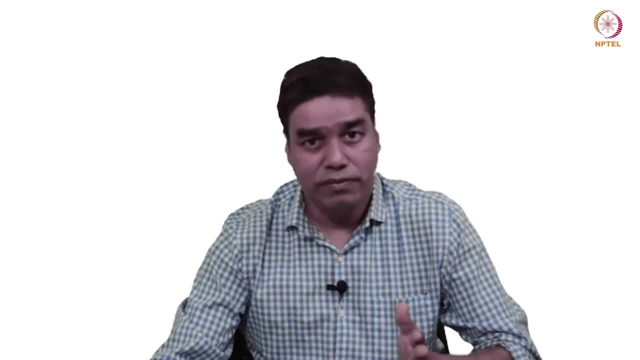 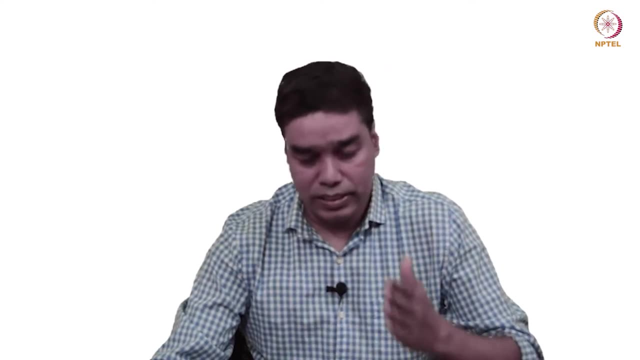 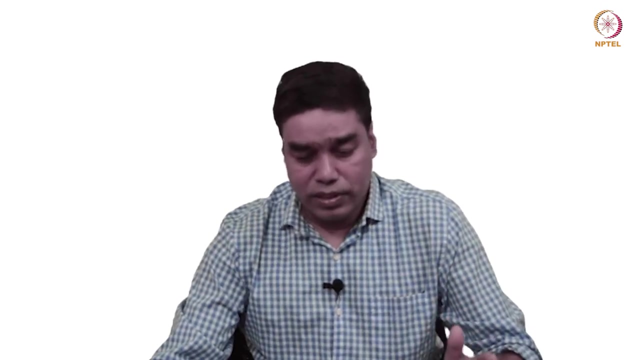 So this is one of the most crucial steps, simply because of the fact that here the final densification will take place, and if something goes wrong in this step, then whatever is done before may all go waste. ok, So therefore, the sintering process. 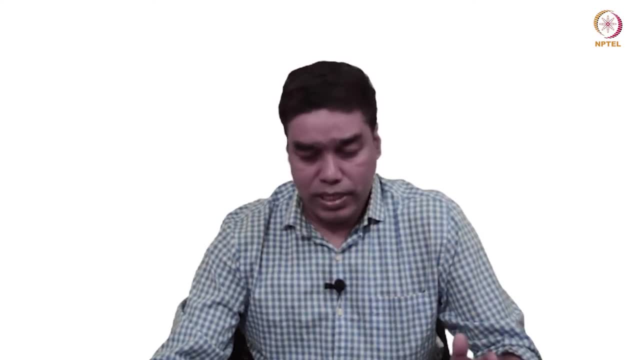 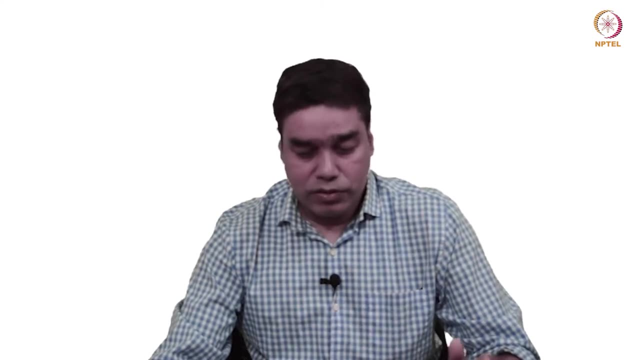 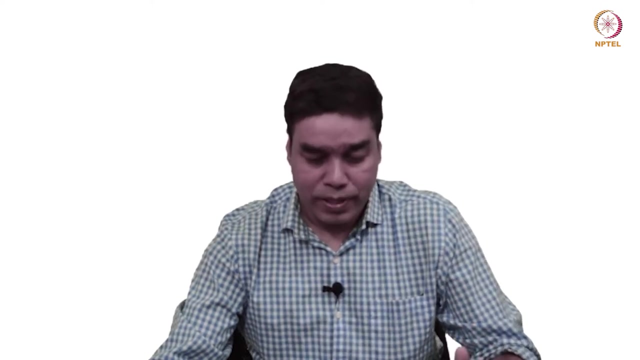 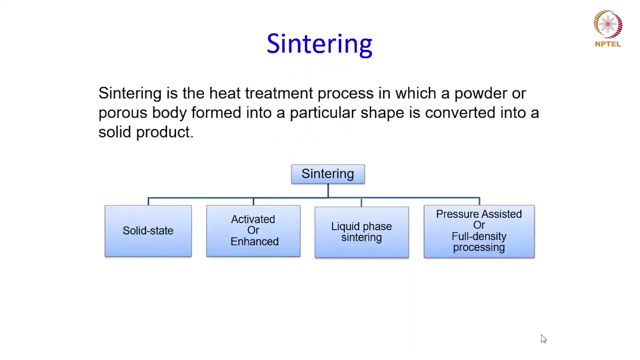 is a very, very crucial step, so much so that sintering in itself is a complete subject, right? So therefore, brace yourself for a series of lectures on this particular topic, starting from today, but let me tell you that will be worth doing, ok? So sintering can be defined as follows. 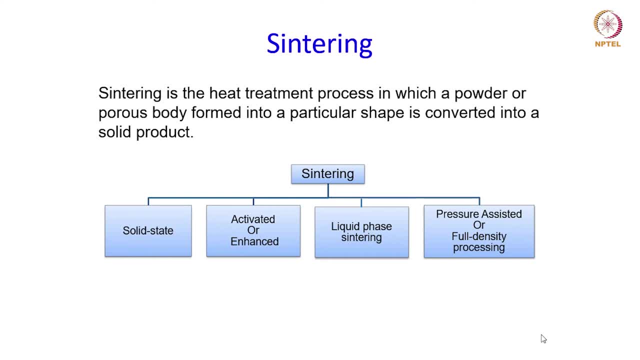 Sintering is the heat treatment process in which a powder or porous body already formed into a particular shape. So this is the process in which a powder or porous body already formed into a particular shape. It means that the mass of powder is converted into a solid product. ok, 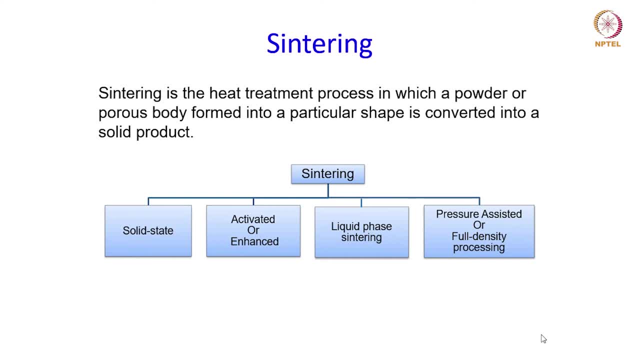 So in the powder metallurgy process, what is done is the都是 powder mass is first compacted and a particular shape is given to it, and then, in order to close all the pores and to densify it, it is heated at a particular temperature for a certain period of time. ok, 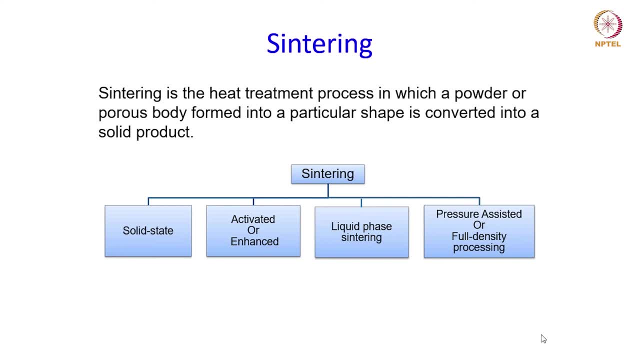 So during this heating process, the densification occurs and at the end of the heat treatment cycle, or the sintering process, a fully dense solid product is obtained. ok, So that is what is called as the sintering process. Now this process can be divided into different categories, as you could see from from here. 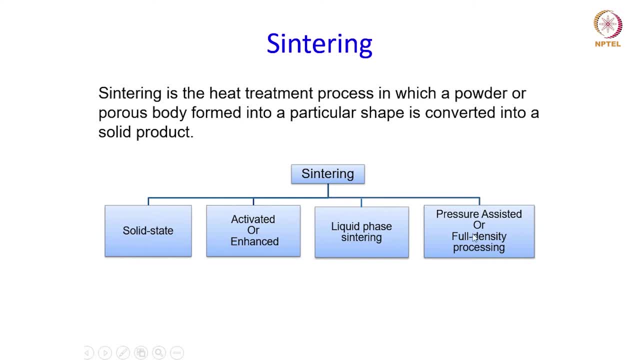 and these are as follows. as you could see from here, Solid state sintering, which is basically sintering a solid mass of powder to densify it And give rise to a solid, dense product. So this happens all in the solid state itself, and you can have some variants of this solid. 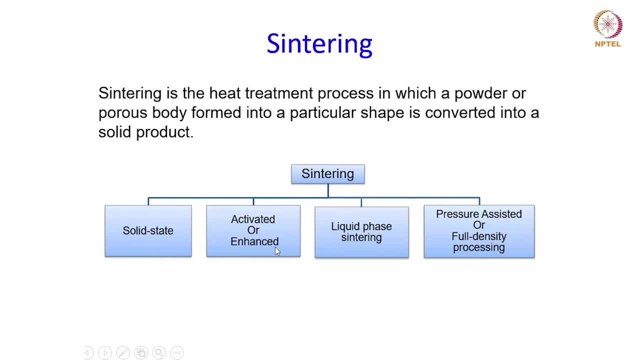 state process. For example, you can have activated or enhanced sintering, in which an agent or an activator can be added to enhance the sintering. or there are some other means also to enhance the dense densification. For example, a phase transformation can be used to enhance it. 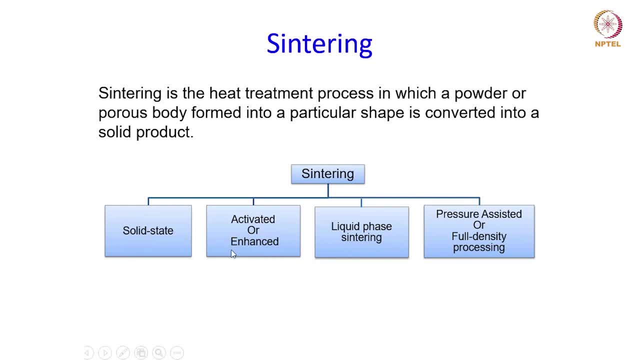 So those kind of processes are known as enhanced sintering, And then, when a liquid phase is involved, that is known as the liquid phase sintering. This is different from the conventional solid state sintering in the sense that, apart from 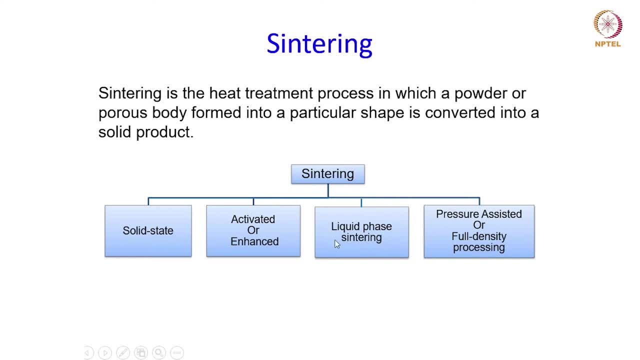 the main solid phase, Solid phase which is to be sintered. there is a second phase which will melt at the sintering temperature, and therefore a liquid phase is also involved in this case. ok, And then, depending on the material, at times the sintering is also done under the application. 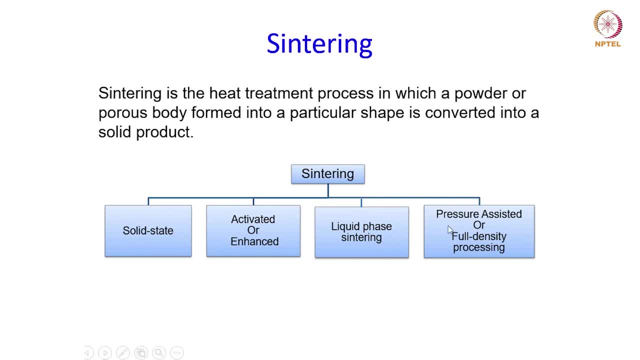 of an external pressure. So those are the pressure assisted sintering. So the pressure assisted sintering is a process of sintering in which a full density is obtained, and therefore these processes are also known as full density processing. ok, 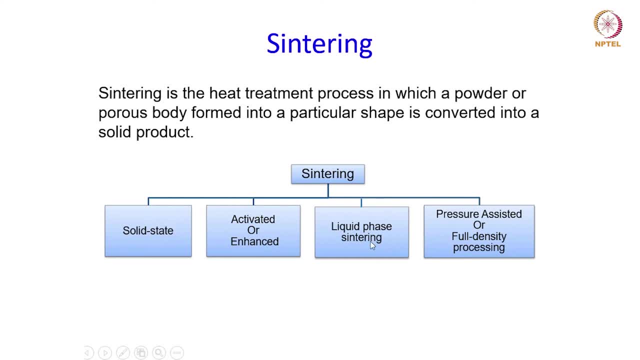 So which method of sintering will be used? that primarily depends on the material which is to be sintered. ok, For example, if you have a material which can be easily compacted and sintered, Then you can use a plastic material which is easily compacted and sintered. 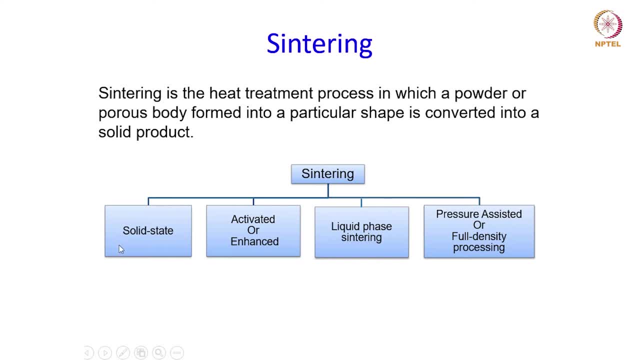 Then you can use a plastic material which is easily compacted and sintered. Then the conventional solid state sintering itself will be enough. On the other hand, you might have materials which are difficult to sinter and you may not be able to get full density by conventional solid state sintering. 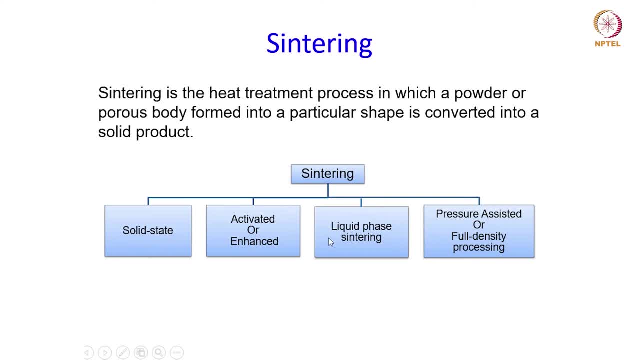 So in those cases you may have to use the other kind of sintering processes, such as the liquid phase sintering or pressure assisted sintering. Then we will talk about the other processes. So we will talk about the other processes. 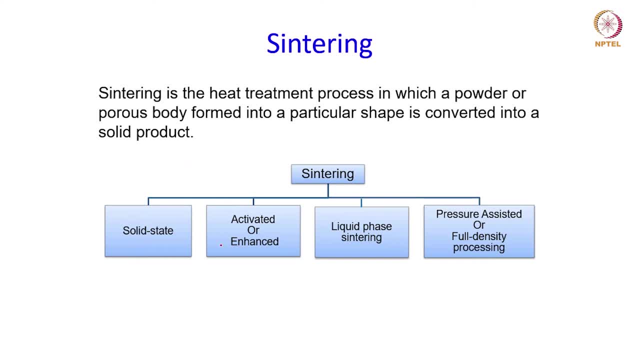 We also have another advanced sintering process, known as spark plasma sintering. This is quite different from all the other sintering processes that we have described in this particular diagram. This is quite different from all the other sintering processes that we have described. 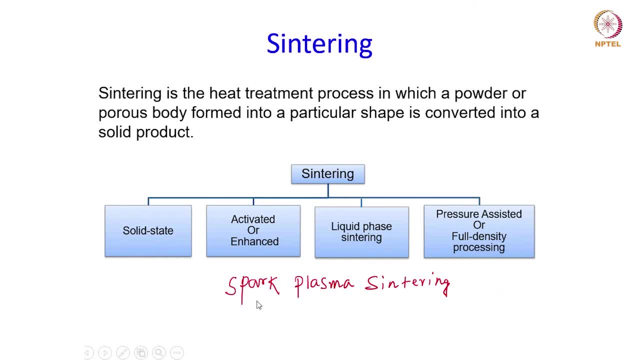 in this particular diagram, In the sense that the heating mechanism in case of spark plasma sintering, or SPS, is quite different from all other sintering processes. right, and due to that, this sintering process is also very effective in sintering hard to sinter materials and the sintering time is. 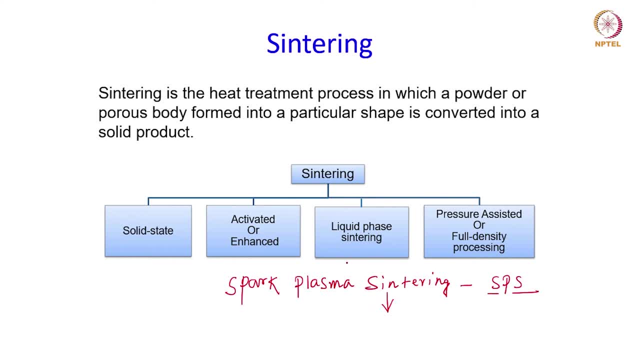 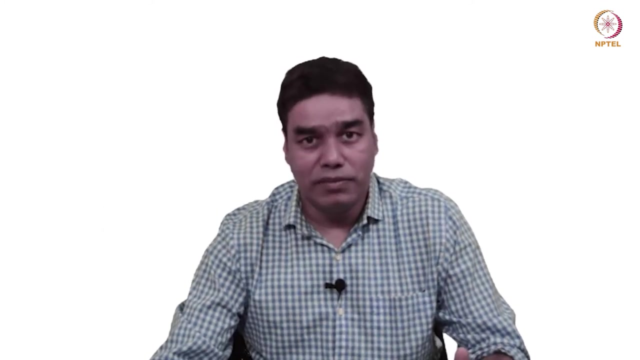 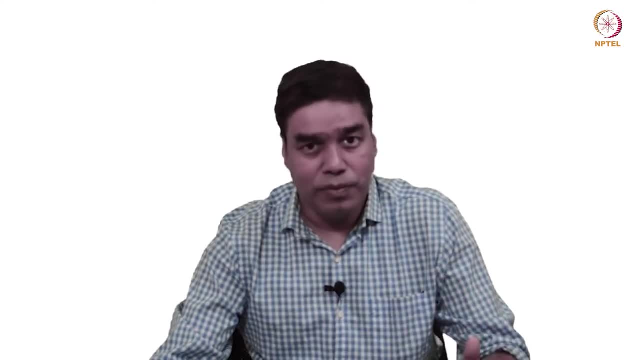 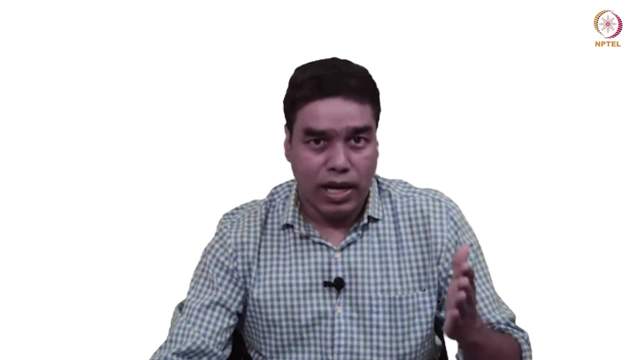 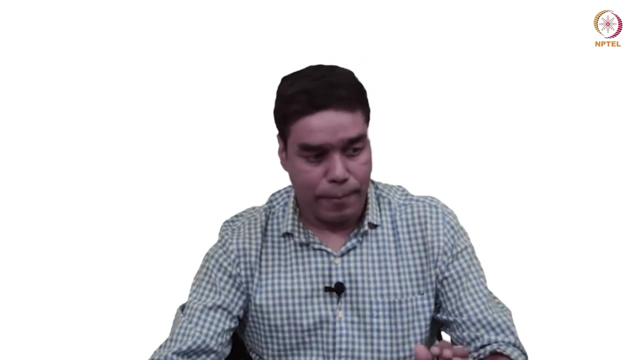 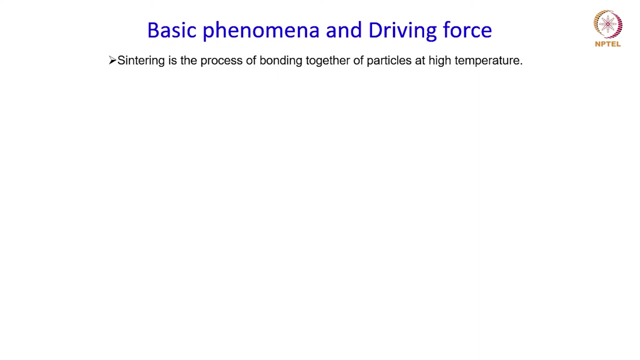 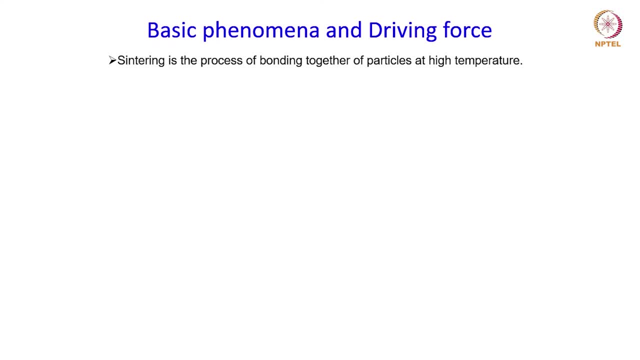 to a particular temperature, depending on the material, because for these pores to be filled, there has to be diffusion occurring, and that will occur only at higher temperatureat higher temperatureWhere the atomic diffusion can happen and the mass can be transported towards the pores, for them to be filledand the densification to take place. okSo now, if you look at that driving, 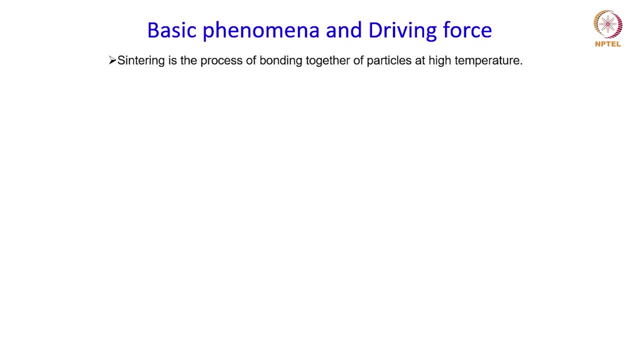 behind this phenomena. first of all, when you heat the compact to higher temperature, there could be two things which can happen. So let us say this is the green compact and the arrangement of the particles. Here you can see that after the compaction process, the particle to particle 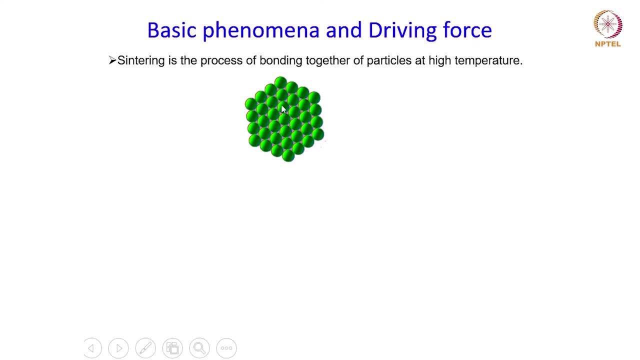 contacts are formed ok, but still there are pores between the particles, and this is what we have discussed before. also, If you remember, we discussed the fractional porosity as it occurs in the green compact and its correlation with the compaction pressure, and so on. So these are the 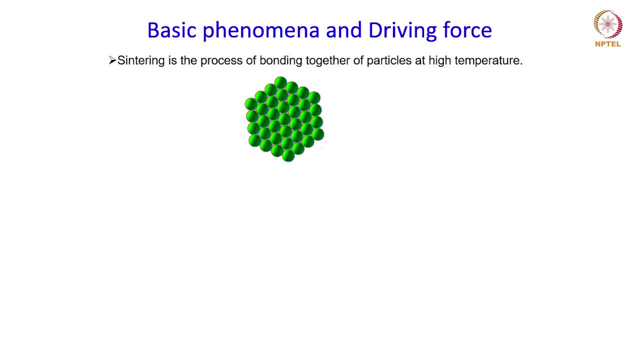 pores which are to be closed for the compaction process. So these are the pores which are to be closed for the compaction process. So these are the pores which are to be closed for the compact to fully densify. ok, So now, as I said, when you heat it to high temperature, two things. 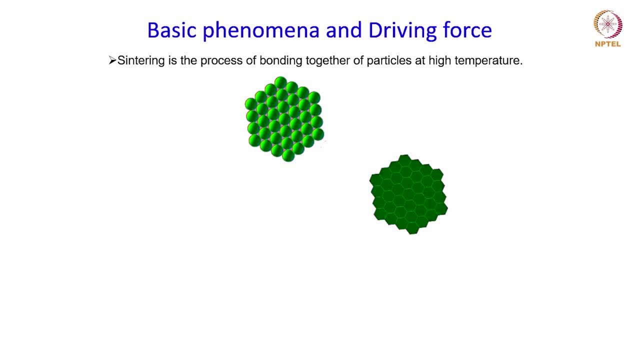 can happen. one: it will densify. where this pores in between, the particles will be completely eliminated and the particle contacts will grow and form. But if you heat it to high temperature it will be completely isolated and it will form this kind of boundaries or form the grain boundaries between the particles. ok, 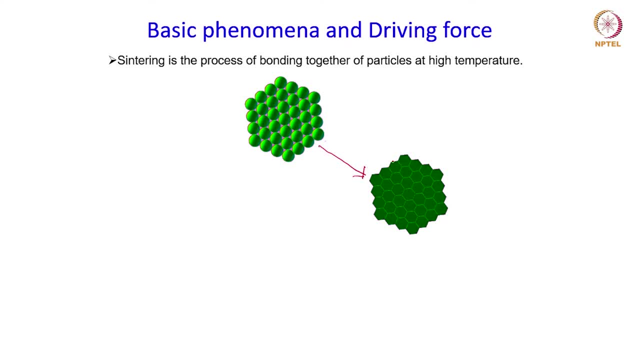 On the other hand, since we are talking about high temperature, it can also lead to coarsening of the particles. ok, Because at high temperature there is a driving force for the growth of the particles as well, as it decreases the total energy of the system, because, as grain growth occurs, number of grains will. 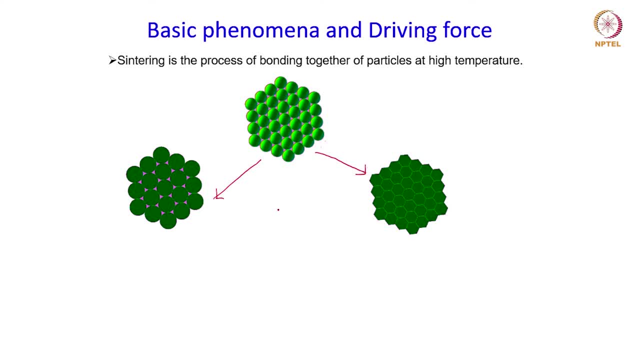 decrease and hence the number of interfaces will also decrease, or in other words, the total grain boundary area will decrease as the grain size increases. ok, So since the interfacial area is decreased, the total interfacial energy will also decrease, and that would lead to a decrease. 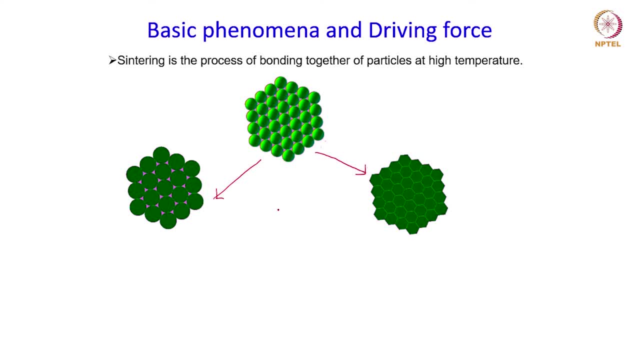 in the total energy of the system. ok, So that is why there is a driving force for the grain growth or coarsening during the sintering process. And when you talk about sintering a porous compact, the pores will decrease. So when you talk about porous compact, the pores will decrease. So 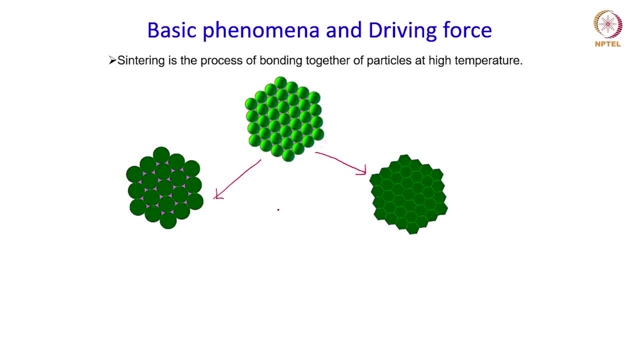 this will also play a role in the grain growth process. So, while talking about the growth during sintering, the pore interactions will also have to be considered because, depending on the locations of the pores- whether they are located along the grain boundaries or inside the grains- 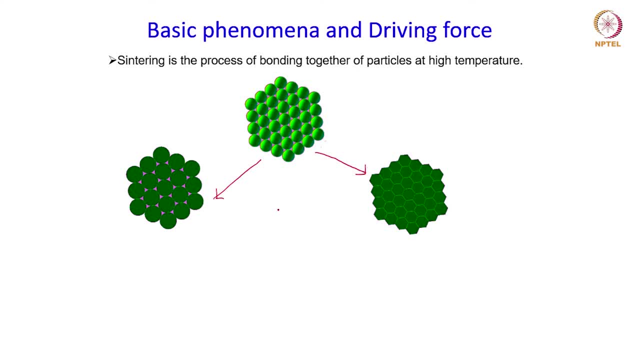 the grain growth behavior will change. ok, The pores are located along the grain boundaries during the final stage of the sintering process, then it is expected that they will retard the grain growth and the grain growth will not be very significant. it will be a normal kind of grain growth. On the other hand, if the pores are located, 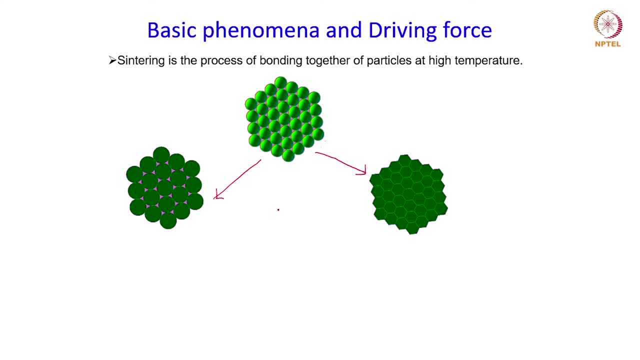 inside the grains, then there is a chance for abnormal grain growth, because now there are no more pores along the boundaries to pin them. So if the pores are located along the grain boundaries and as a result of that, the grains can grow abnormally, ok. So the occurrence of grain 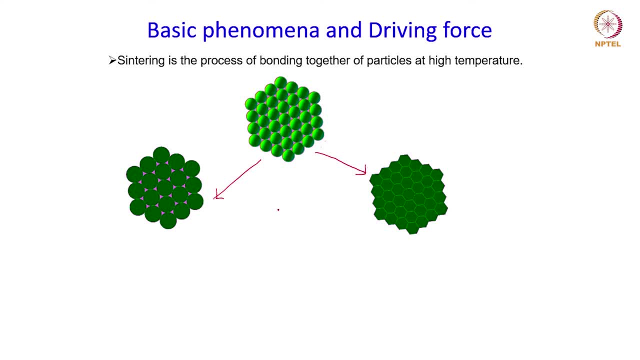 growth or coarsening during sintering is quite normal. So therefore, apart from densification, coarsening will also occur simultaneously. So again, this is an example of the coarsening process in the compact, So as more interfaces are generated because of the densification process, 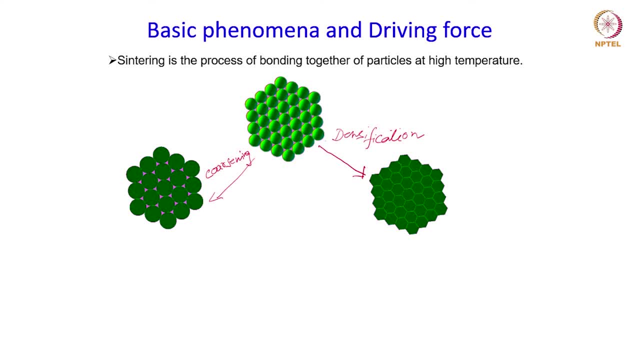 the interfacial energy will change. So if gamma is the specific interfacial energy, then the change in the surface energy or interfacial energy due to densification will be this And due to the coarsening, the area is going to change and due to that, 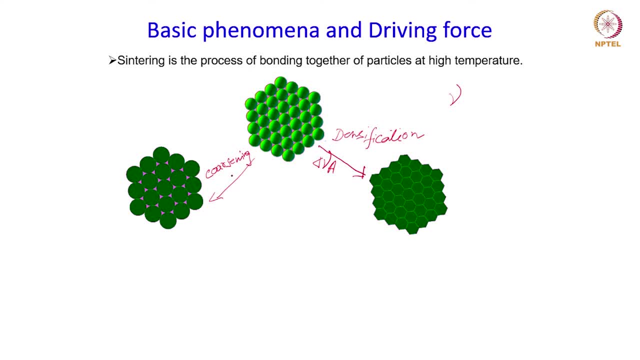 the change in the surface energy will be So gamma into delta A as opposed to delta gamma into A for the densification process right. So the total change in the surface energy will be coming from these two contributions, one from the densification and the other from the coarsening right. 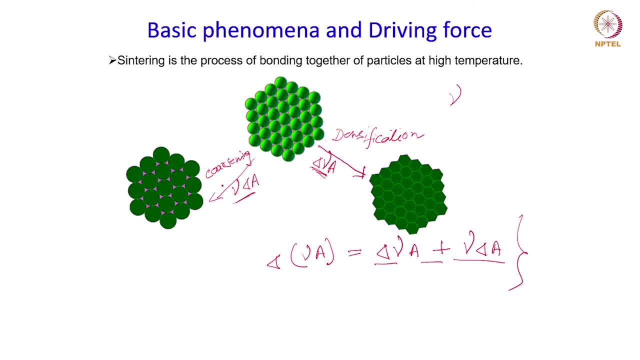 So this process of densification and coarsening will essentially lead to a decrease in that total surface energy of the system. ok, So when sintering finally occurs in the sintered compact, both of these phenomena will take place. ok, And 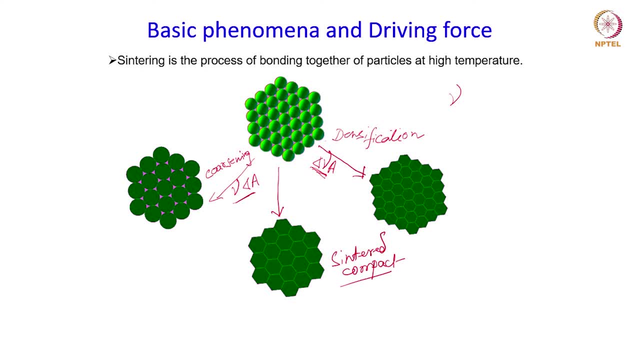 that can be seen from this diagram as well. Here this is the demonstrator- with just two particles, both having equal diameter D. So this is the contact which has formed during compaction And as the compact is sintered, a neck will form. 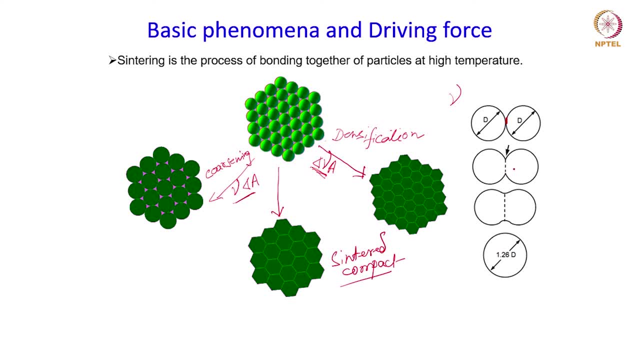 in these contact points and as the sintering proceeds, this neck will grow, and as it grows, the solid vapor interface will be replaced by this. So these are the crest of this system. ok, Now let us use the диablo or その snk here. to simulate a solid vapor interface. This would look like this. So, afterurdist having thick particles being formed in the system, they will also be able to shorter depth. OK, In fact, throughout the these tests of solche sono actuarial supercell did a keen efforts until the 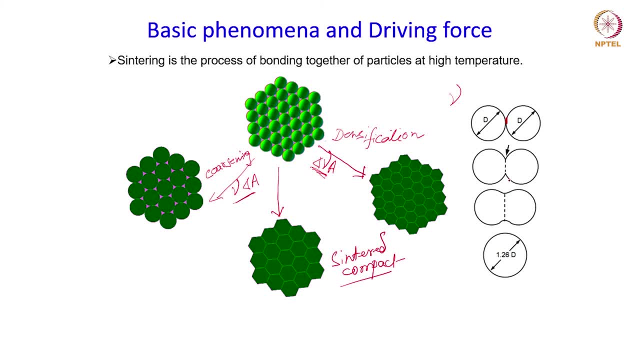 sim einfoto of attention. is не 분� purl also done, But those points of surface energyён't bear great. the solid-solid interface, which means that the grain boundaries will replace the solid vapor interfaces. ok, And this final picture of a bigger particle that you see over here. that depicts the 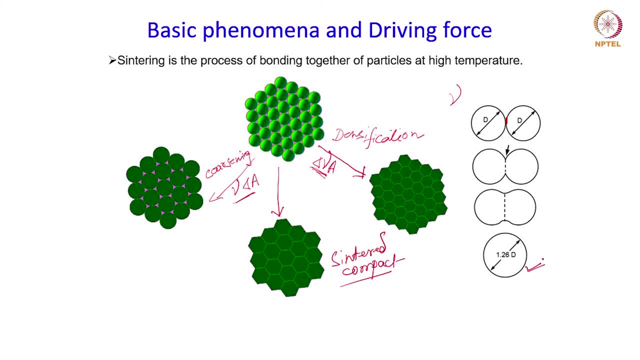 coarsening process wherein, if sufficient time is allowed, these two particles of diameter d can coalesce into one particle with a bigger diameter, right? So that is the coarsening process, right? So, as I said, you can see here also how the sintering process involves both densification. 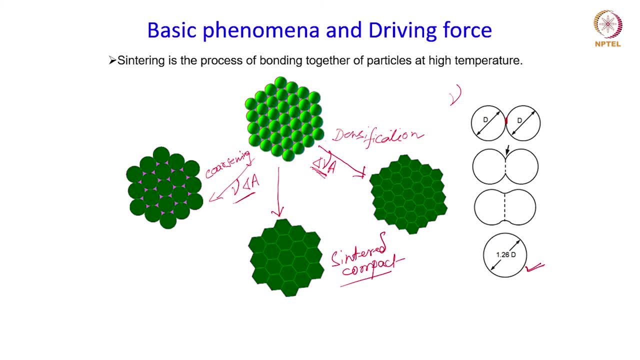 as well as grain coarsening. So therefore, the total change in the surface energy delta gamma a will be given by these two contributions, one from densification and the other from coarsening right. So this phenomena that takes place during the sintering process, 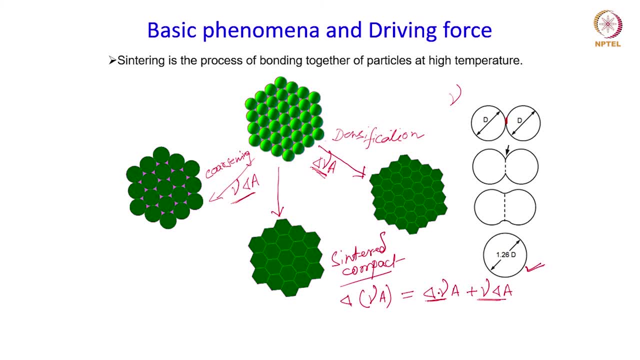 it basically leads to a decrease in the total surface energy of the system, and that is what drives the process. ok, So therefore, we can say that the driving force for the sintering process is the reduction in total surface energy. ok, Now, if you look at the process as to: 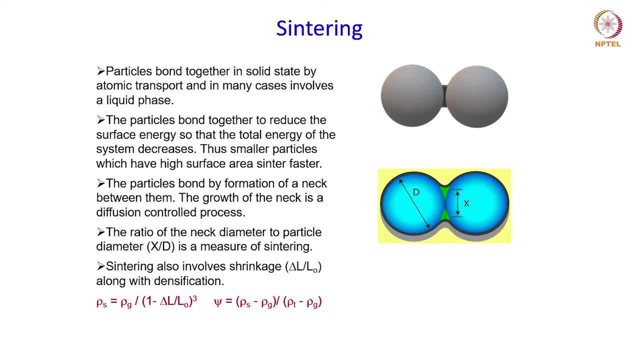 what happens, you know. first we can just see two particles as to how do the bond when they are heated to a particular temperature for the sintering process. So let us say we are having these two particles which have formed a point contact during the compaction process and, as it is heated, now for 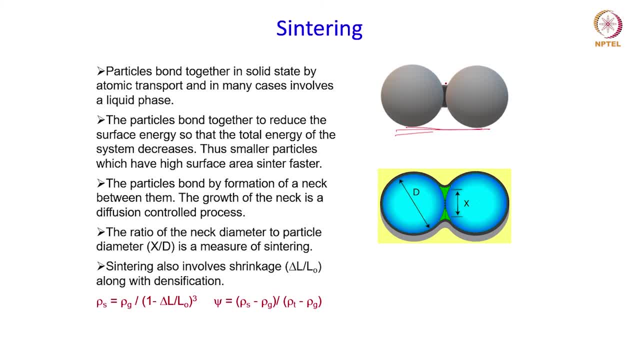 the sintering process. So this is the contact during the compaction process and as it is heated now for the sintering process, This contact will grow in the form of a neck right. So a neck will first form between the particles at the contact points and this neck will grow by diffusional transport of 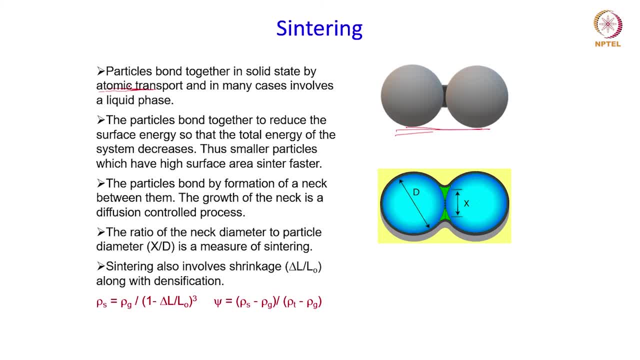 matter or atomic transport, and in some cases it can also involve liquid phase. So this bonding of particles will reduce the surface energy, as I said before, So that the total energy of the system decreases. and therefore you can also say that smaller particles, which 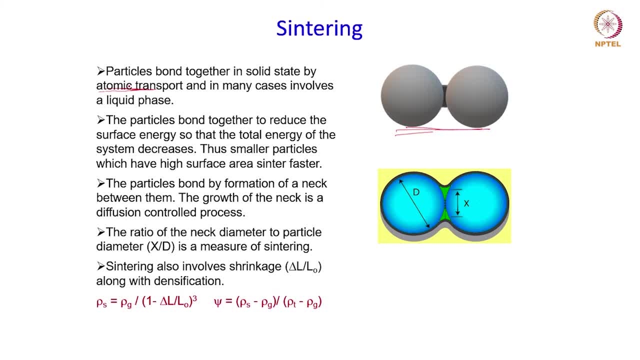 have higher specific surface area will sinter faster compared to larger particles, right? Because if the surface area is higher, it will also have higher driving force for the sintering process. So, as I said, the particles will bond by formation of a neck between them, As you see over here. this is the starting. 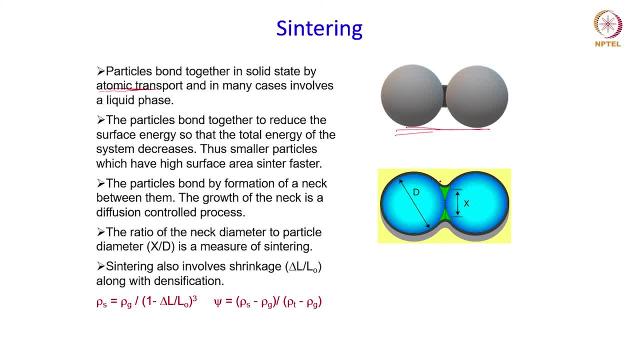 of the formation of the neck, and it will form in a manner like this, as it is shown schematically in this particular picture over here: And the growth of the neck is a diffusion control process, right? So the mass transport has to happen at towards the neck for it to grow and the pores to be closed, and that ultimately will lead. 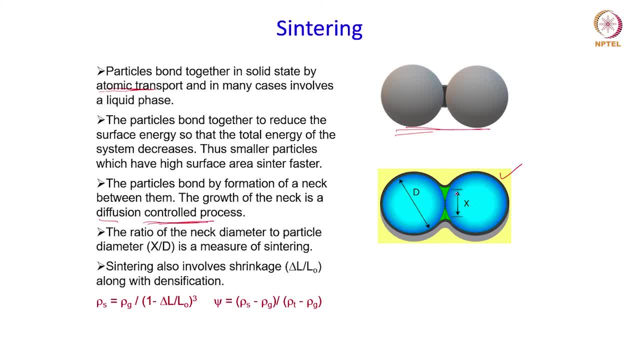 to densification. So here there is a neck radius, as you could see, which is written as x, and the ratio of the neck diameter to the particle diameter, x by d, is a measure of the sintering, As to what extent the particles have sintered. we. 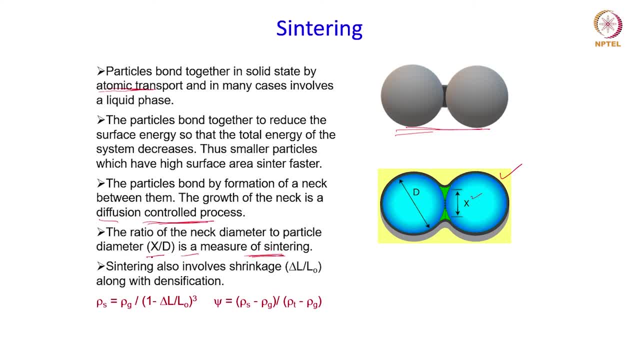 will determine by using this X by d ratio. Now, as we have seen in this group, we will have x and d ratio in the center pan, or decided size ratio can be. that can be guessed by looking at this X by d ratio. ok, And in sintering, as you would have already, 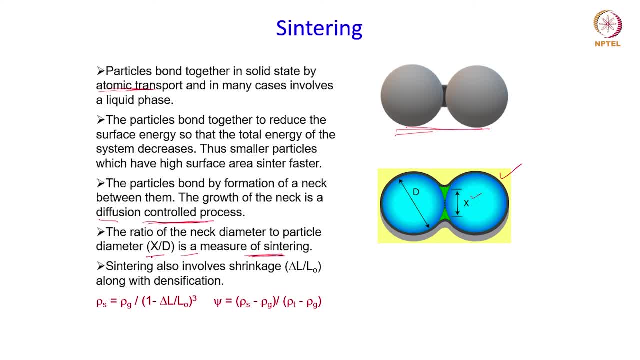 understood by now. the pores are closing, so that means, you know, the particles are coming closer and closer, which is given by delta L, by L naught, where delta L is the change in the dimension and L naught is the initial dimension. ok, So this can be one of those dimensional parameters. 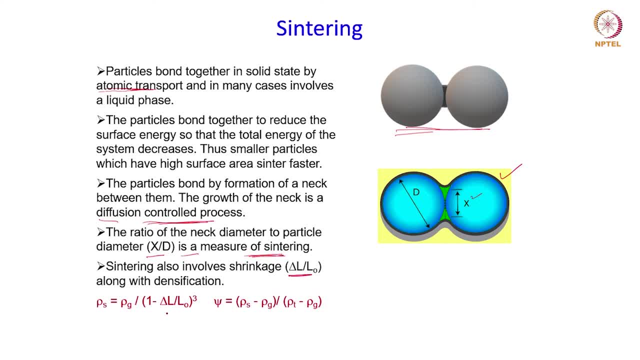 for example, the length ok. And this shrinkage is related to the sintered density rho s, ok and the green density rho g with this equation. So from this relation you can say that the compact densifies from the green density rho g to the sintered density rho s, which is higher compared to rho g. 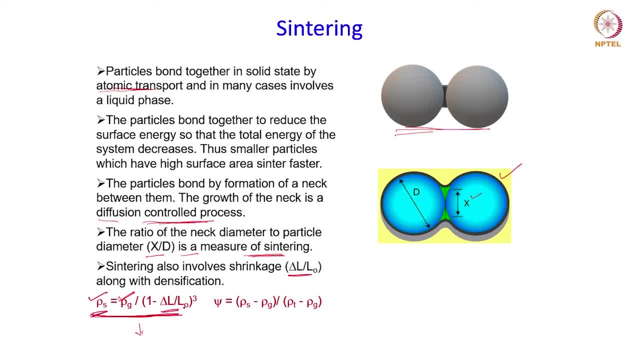 due to the shrinkage which takes place during the centering process, right? So densification will be always accompanied by shrinkage, ok, And the densification parameter, psi, is given by a relationship like this. So this is basically the ratio of 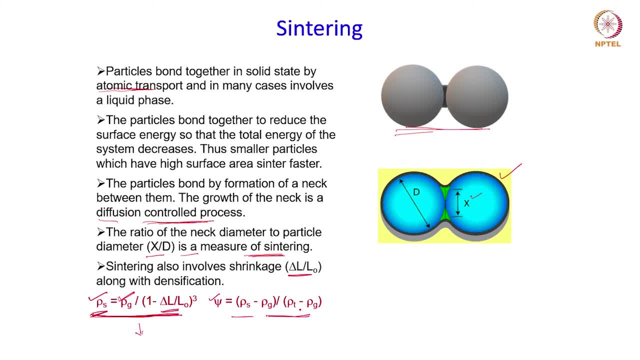 the change in the density. that means rho s minus rho g, the density of the sintered compact and the green compact, the difference of that divided by the change needed to attain a pore free, solid, So rho t here in the denominator is the theoretical density of the material. 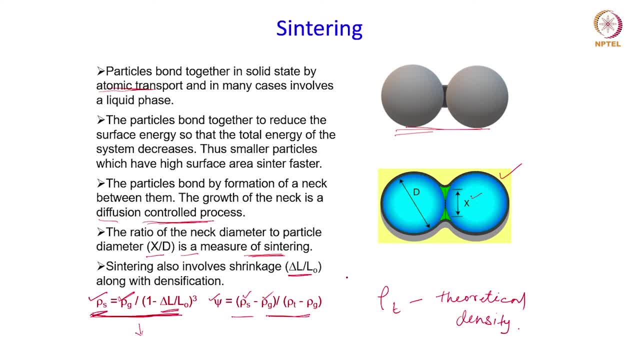 ok, So that is how the densification parameter psi, is defined. Ok, So densification is all about elimination of the pores And the final density, the neck size, surface area and shrinkage. these are all related to the measures of the pore elimination process which takes place during sintering. 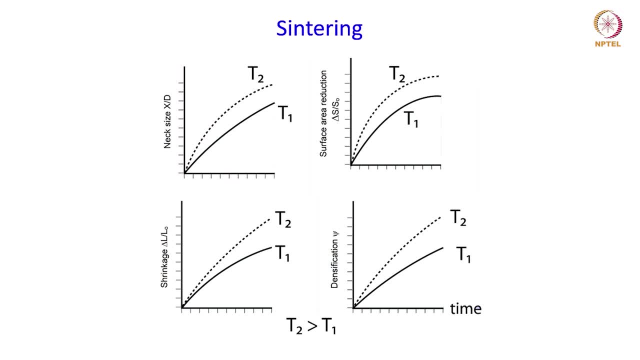 And, as I said, sintering is a high temperature process For all these phenomena that leads to elimination of the pore. a higher temperature is needed because the atomic diffusion that happens, that is, a thermally activated process, and therefore for the densification to occur, the 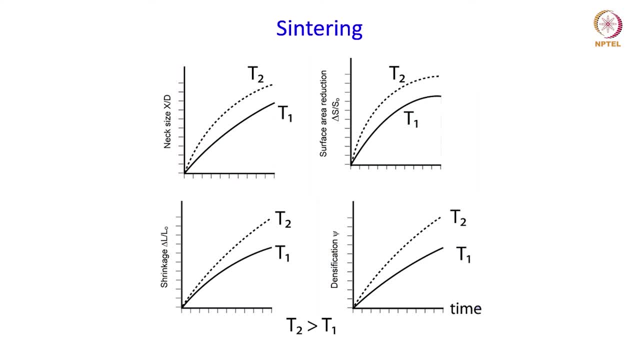 compact has to be used. So the densification of the pore is a high temperature process. So the densification of the pore is related to higher temperature And through these plots the effect of temperature can be seen. Here T 2 is greater than T 1,. 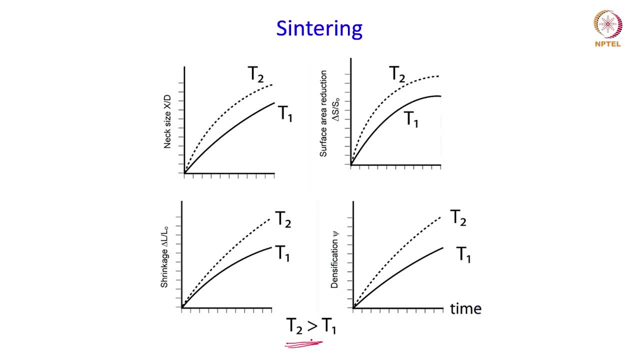 T is the temperature right. So this is depicted in terms of the densification parameters, or the parameters which can be related to the densification, such as the neck size, the surface area reduction, delta S by S naught, the shrinkage and the densification parameter. 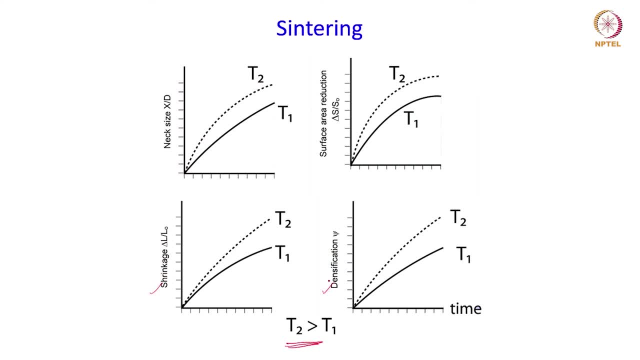 that we defined just now. ok, So here you can see that as the temperature is increased, the densification is also increased, because all these parameters which define densification increases with increasing temperature Because, as I said, the processes which lead to pore closure are all thermally activated processes and therefore, 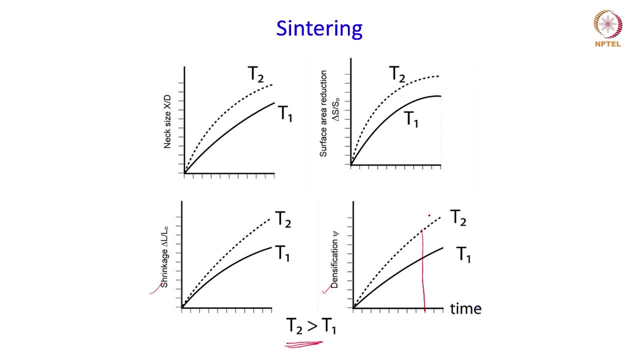 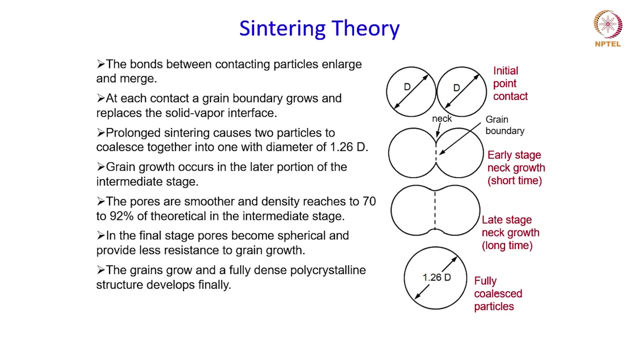 an increase in the temperature will lead to a higher densification. So when you talk about the sintering process as such, the two important parameters are the temperature and the time. ok, So now coming back to this bonding process. So 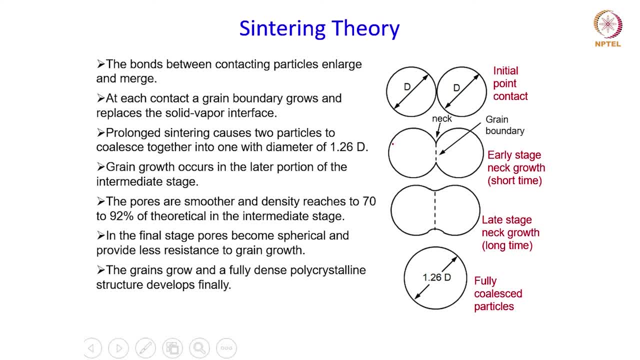 So, So. So this, again you know, depicts the sintering process as it proceeds, starting from the development of the neck at the contact points during the early stage of sintering and then, as the process continues, this neck grows in the later stages when more time is allowed during the sintering. 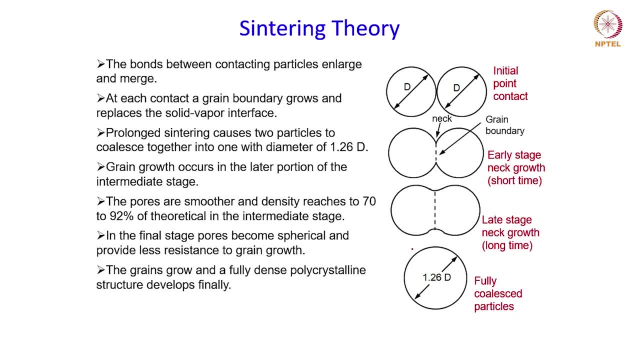 at a particular temperature, and if it happens for a prolonged period of time, then the particles can also coalesce to bigger size. Now, for all this to happen, the matter has to be transported to the neck, for it to grow and for the pores to close. 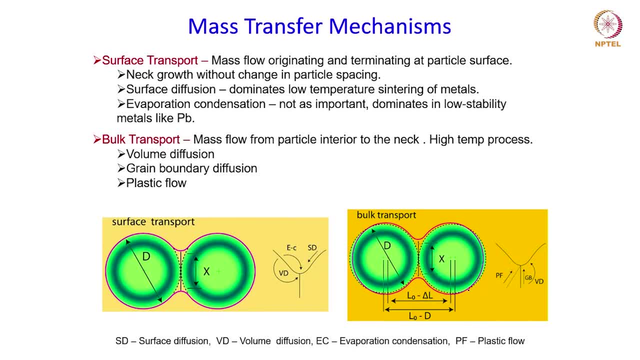 So this atomic diffusion occurs through well defined paths. Those diffusional paths are Depicts are depicted in this diagram over here. These are basically the surface diffusion, the volume diffusion, which is one of the bulk transport processes. Then you also have grain boundary diffusion, where the transport of the matter occurs along. 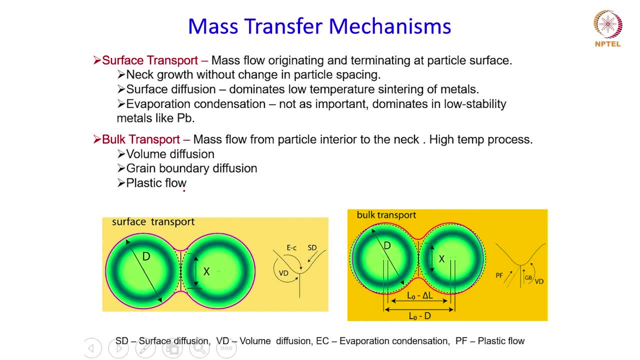 the grain boundaries, and then you have plastic flow- ok. And there is one more type of mechanism known as Evaporation, condensation, that can also happen, for the matter. transport towards the neck- ok. So here you can see, diffusion plays a very important role for the densification to occur. 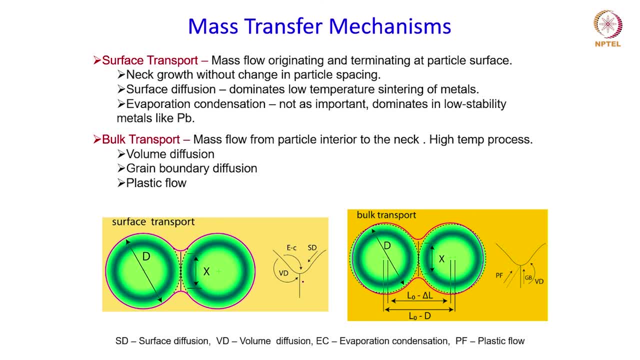 during the sintering process And therefore at this point it will be good to have a little bit of discussion about the diffusion phenomena as such gens thu. 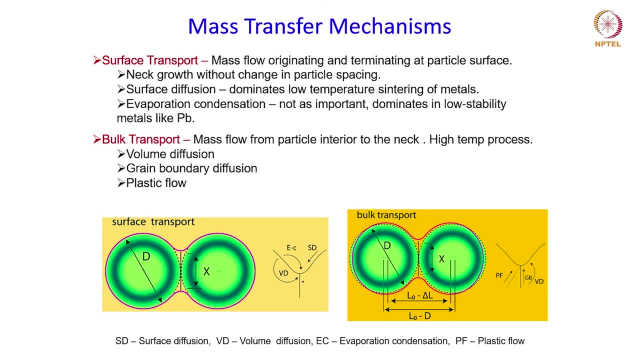 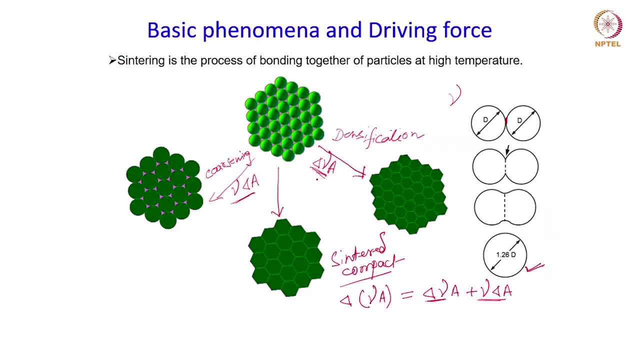 this particular lecture. this is all I have, but before we close, let us take a moment to summarize the lecture. So today we talked about the basic principle of the centering process and we have learned that the main driving force for the centering is the reduction in the total surface energy that leads to an ultimate reduction in the 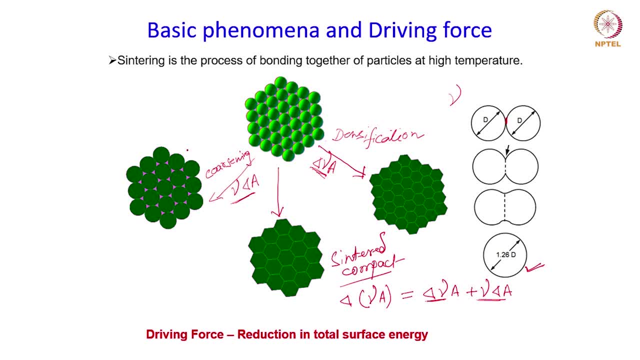 total energy of the system. And the centering process basically starts with the formation of a neck at the contact points of the particles and as it proceeds, the neck grows, which ultimately leads to pore closure. ok, So therefore, the neck ratio, which is the 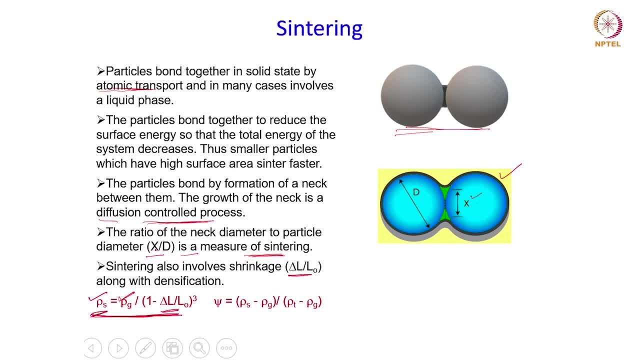 ratio of the diameter of the neck to the diameter of the particle is taken as the measure of the centering, And centering is always associated with shrinkage. So whenever densification occurs, shrinkage will be accompanied and therefore the shrinkage also is an indication. 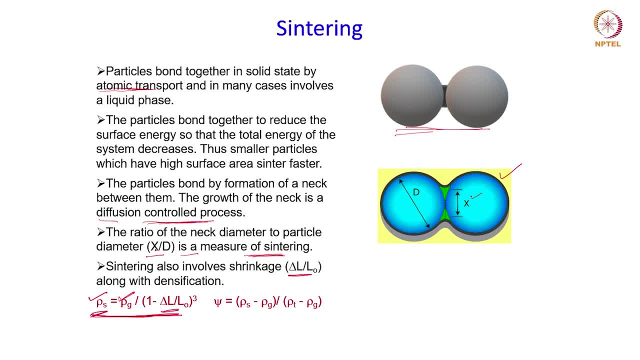 of the densification which occurs in the centering process And therefore the sintered density and the green density- that means the transformation of this compact from the green density towards the higher sintered density- is related to the through this particular relationship over here. ok, And then we defined a parameter called 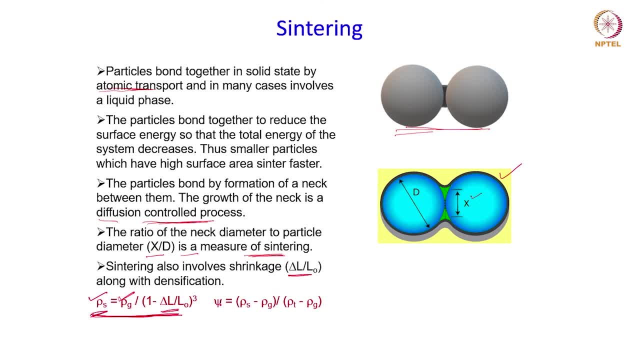 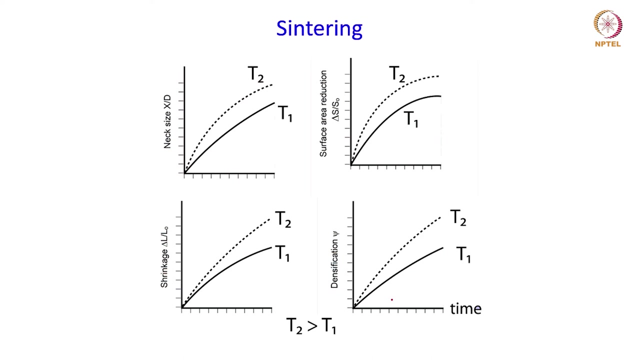 the densification parameter, which is related to the final density which has to be achieved at the end of the centering process. So this is the densification parameter written as psi. and then we talked about the effect of temperature on the sintering. The phenomena which happens during the sintering process is thermally. 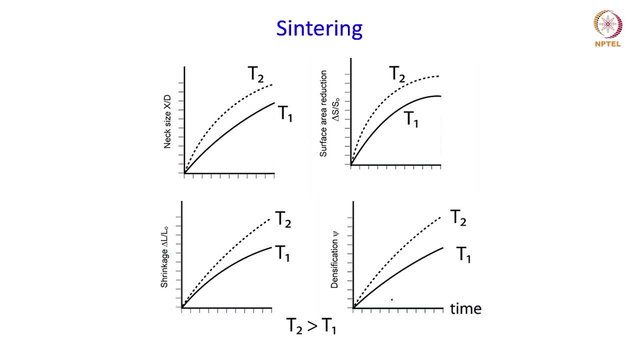 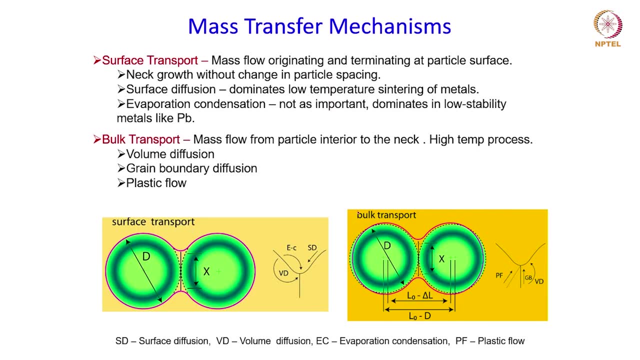 activated and therefore any increase in the temperature will lead to a higher densification during the sintering process. Then we started talking about the diffusion mechanisms, or different paths of mass transport that you have in case of the sintering process. So these are basically categorized into two different categories. one is the surface transport. 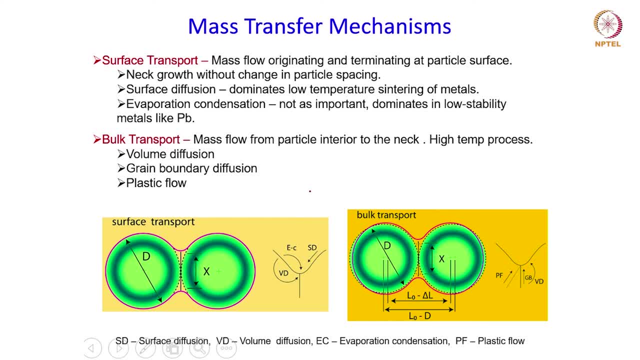 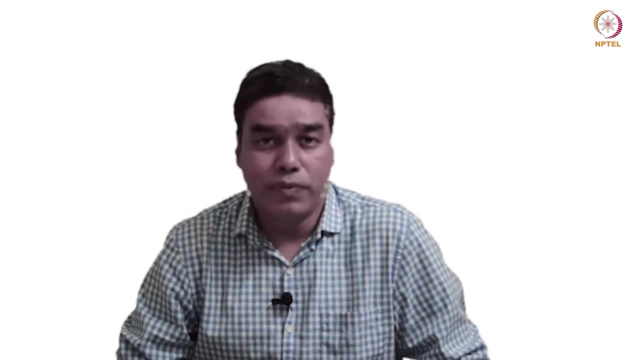 and other is the bulk transport, ok, And this mass transport through all these different paths ultimately leads to the densification which takes place during the sintering process. ok, So with that we come to the end of this class. Thank you for your attention. you.